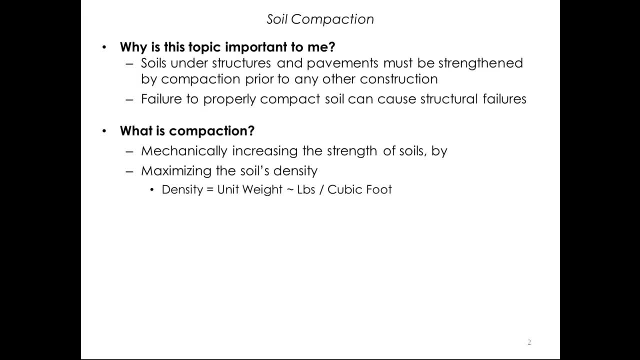 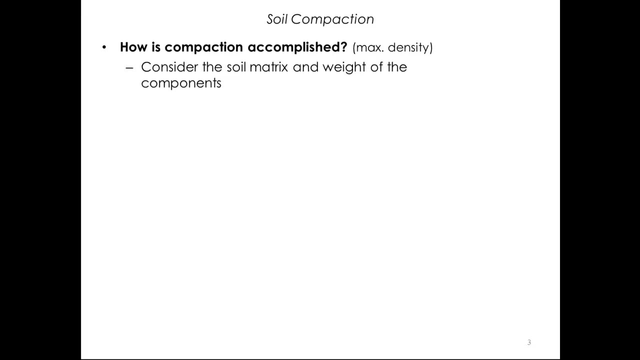 base their design work on some uniform soil bearing value, A bearing value that the site development contractor must achieve by the proper compaction of the soils. In order to understand how compaction is achieved, let's review the compaction of soil. As you may have learned in another one of these videos, soil is a matrix of three constituents. 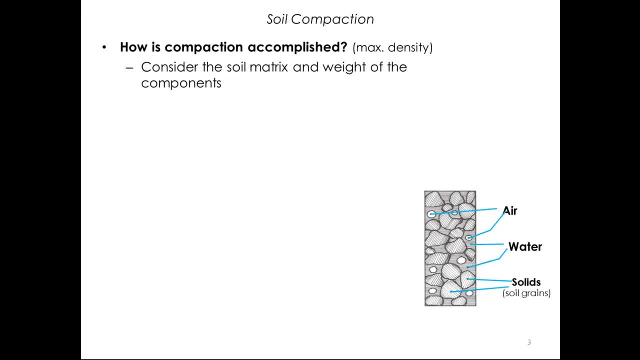 solids or soil grains, air and water in some combination, which is illustrated here. Sometimes, a phase model is also helpful. The non-soil spaces in the matrix are known as the void spaces, and that space is filled with air and water in some combination, Since the goal of compaction is to make the soil heavier. 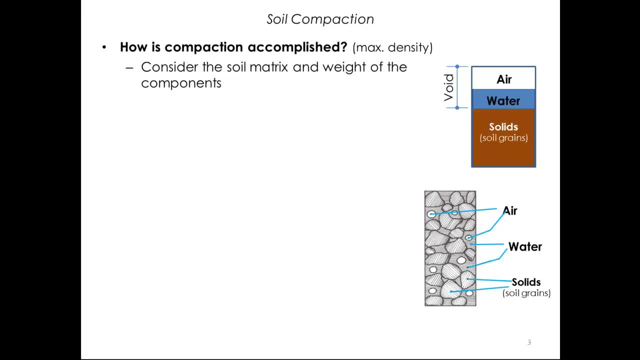 more dense. we need to be aware of the weights of these three constituents. You may remember the concept of specific gravity from high school. It is simply the comparison of the unit weight of something to the unit weight of water. So, as we see here, air has no appreciable. 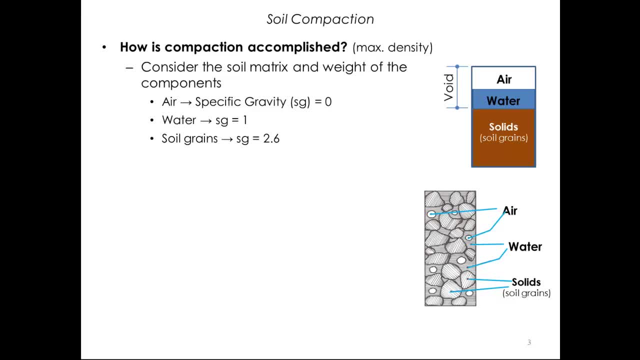 weight, and soil particles are about 2.6 times heavier than a like volume of water. This has an implication in the context of what is in the void space. Now. keep in mind that soil grains are nothing more than very small pieces of rock, and they are not reduced in size by the 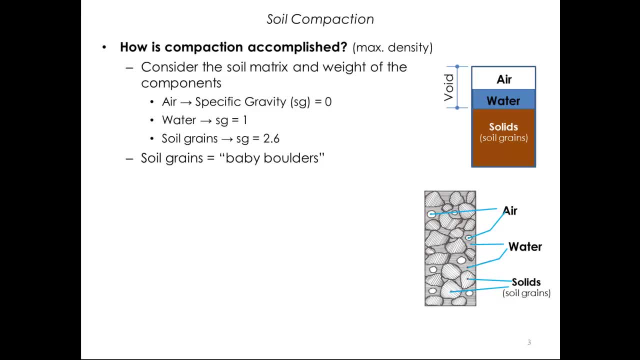 compaction process. The process of compacting is about reducing the size of the void space by realigning the soil grains into a more dense arrangement and filling that remaining space with the heaviest possible material of our three constituents. Since not all possible void space can be eliminated, the second best alternative after grain- 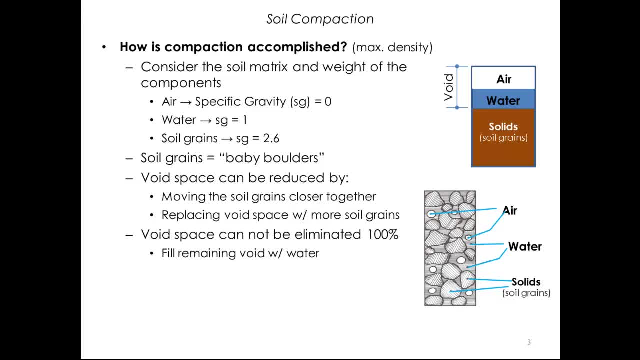 alignment is to fill that remaining space with water. So to answer the question again, compaction is accomplished by applying energy to the soils with heavy equipment to realign the soil grains in a more tightly packed pattern and by adding just enough water to fill the remaining void. 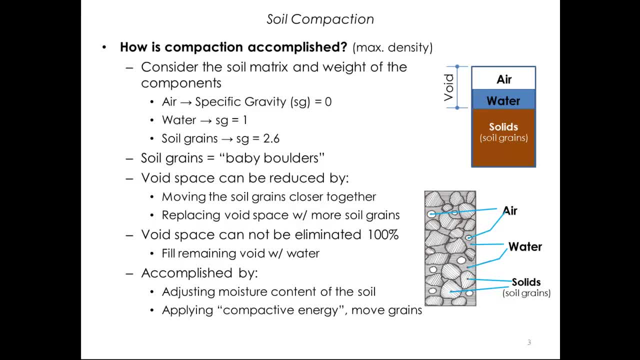 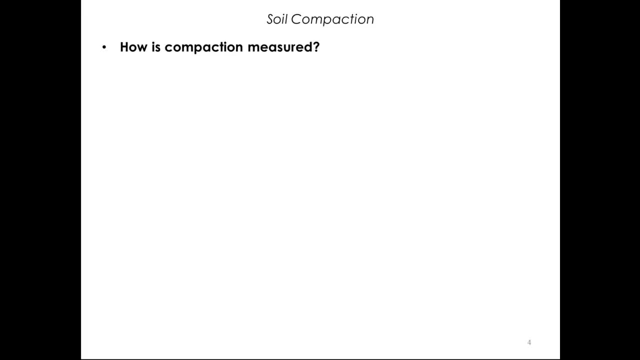 spaces. Now that we have some understanding of how compaction is achieved, let's understand how it is measured. There are standardized ASTM tests used to determine the maximum, that is, the theoretical density, of any soil type. As you see, the history of this test goes back to the 1930s and the test is named after its 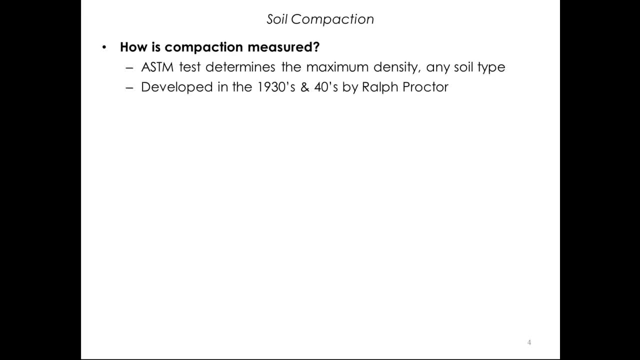 inventor Ralph Proctor. Proctor's work identified the important role that water plays in the compaction process. Let's drop back in our discussion again to the three constituents of soil for a minute. We understand that after grain realignment we need to fill the remaining 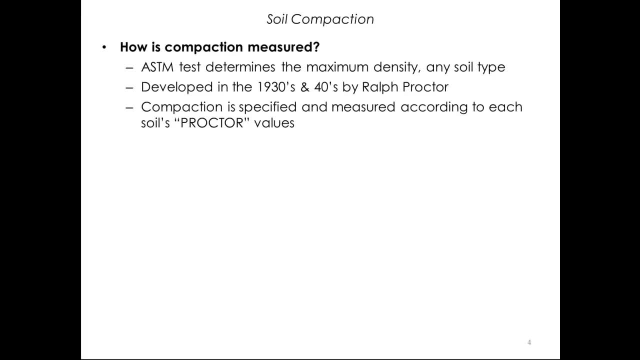 void space with water for maximum density. right, But the key point here is that, since water doesn't compress, if we have too much water it will displace soil grains and make the soil less dense. Remember, the specific gravity of water is one and of soil is 2.6.. This is pretty neat. 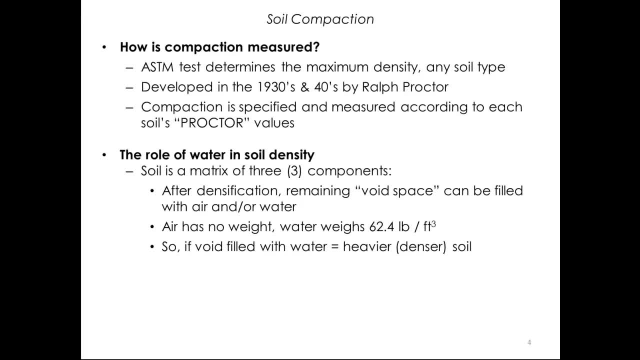 If we don't have enough water, the soil will be less dense than it could be, and if we have too much water, the soil will also bend easier and faster. the soil will be less dense than it could be dense than it could be. What this illustrates is that there is a direct relationship between soil. 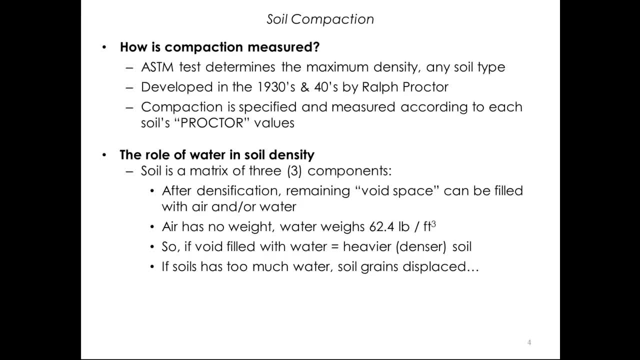 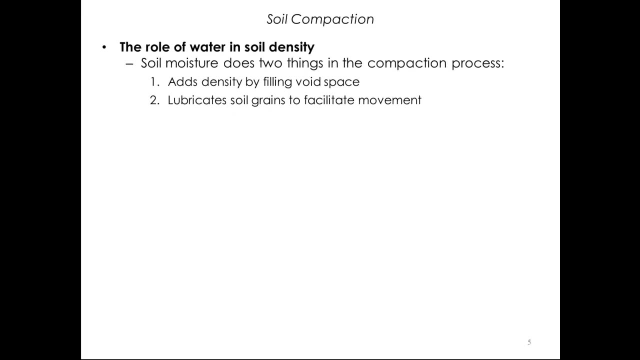 moisture and soil compaction. In fact, another name for the proctor is the moisture density curve. Let's explore the idea of the moisture density curve a little further. Just a quick recap: We understand how water is better than air in the compacted soils. void space, A second benefit of 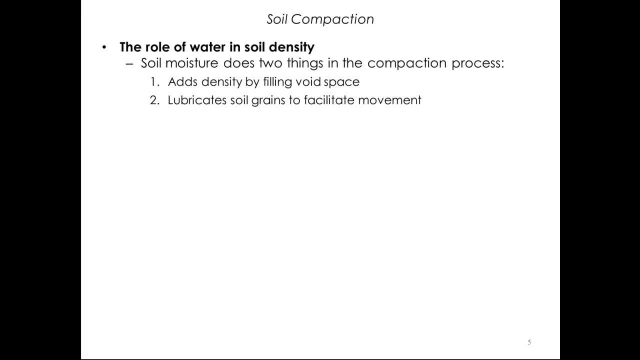 the water is that it acts as a lubricant as we apply the compacted energy needed to realign the grains. Okay, now to the concept of the curve. We said soil compaction is a process of increasing the density or unit weight. So on the left we see a simple graph with density and moisture. 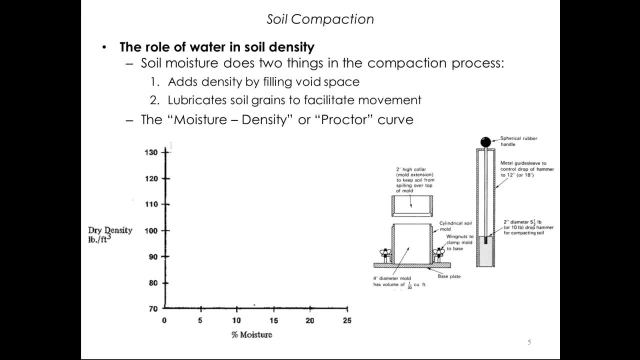 content, as the two axis On the right is equipment used to run the proctor test. What happens is the mold is weighed empty and then the collar is attached. A fairly dry sample of soil is placed into the mold in three separate layers, and each layer is compacted with 25 blows from the drop hammer. 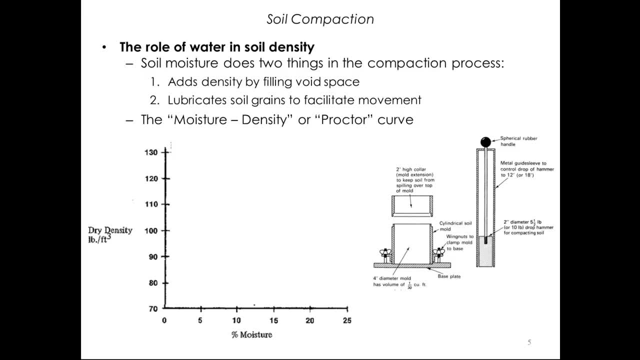 After all, material is in the mold. the collar is removed, the soil is trimmed off and the filled mold is then weighed. After weighing, a small sample of the soil is removed and tested to determine the percent moisture in the soil. The corrected dry weight of the soil in the mold is then plotted on the graph represented by this red X. 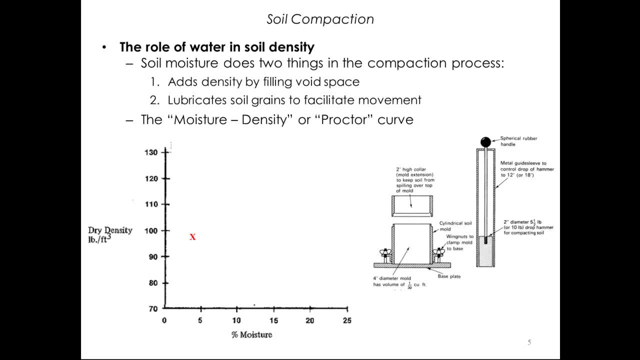 Say, at about 97 pounds and 4% moisture. The soil from the mold is then mixed with a little more water and the process is repeated. and another point is added to the graph Notice at this point, because of the additional water, has a higher density. 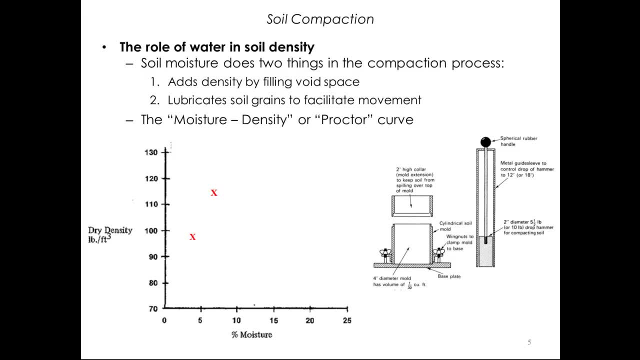 The process is repeated a third time, with the addition of even more water, and another point is plotted which is still heavier than the earlier plots. Again, the process is repeated a third time. Notice: at this point, because of the additional water has a higher density. 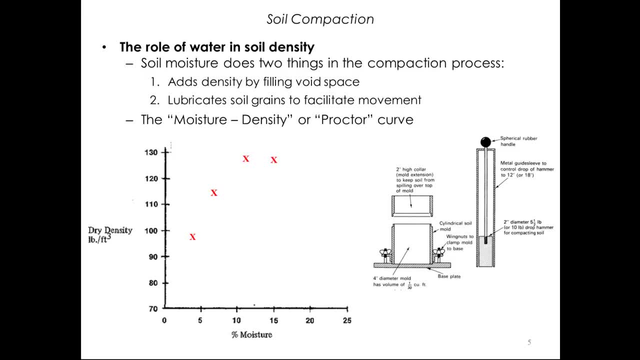 The process is repeated a fourth time, with even more water added and the next point is plotted. However, notice what happened this time. Why did the last plot weigh slightly less than the previous one? The answer is: the higher percentage of water has now started to displace soil grains. 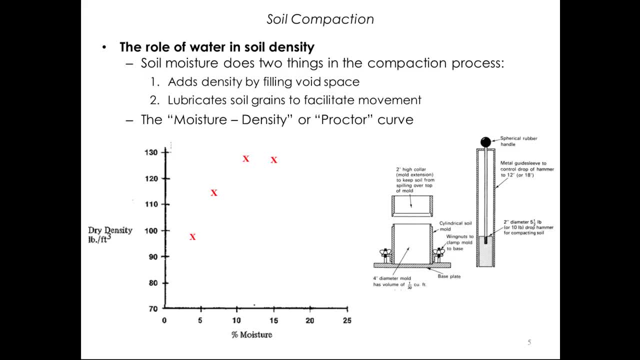 So we just traded soil at a specific gravity of 6 for water at a specific gravity of 1.. Okay, probably one or two more molds are made with more water added and the points plotted. Then the points are plotted, Then the points are connected and we have our proctor or moisture density curve. 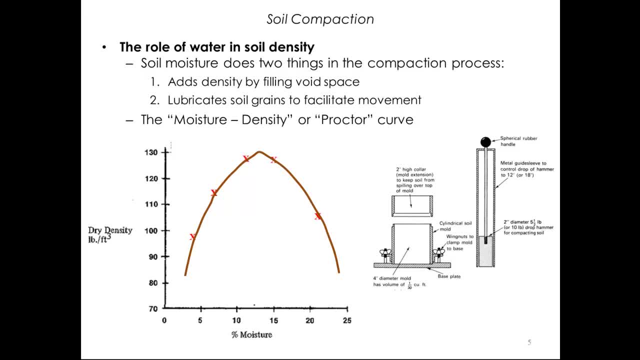 The curve clearly indicates the relationship between moisture content and density, but only for this particular soil sample tested. Let's learn two more terms in regard to soil compaction. If we plot a horizontal line from the very top of the curve like this, we call that value, which is about 130 pounds of cubic foot in this case. 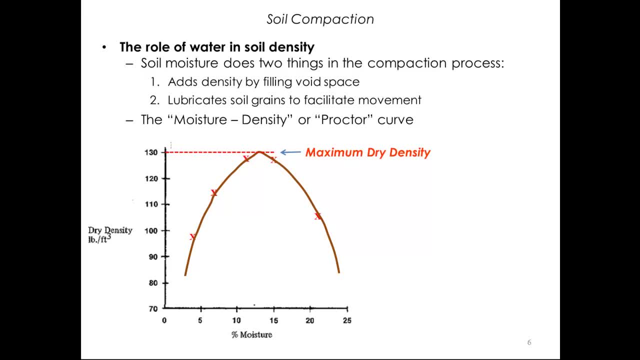 dry density. In other words, this is our theoretical maximum density for that soil under the Proctor test. Next, if we plot a vertical line down from the very top of the curve to intersect the moisture content axis, we find what is called the optimum moisture content. This is 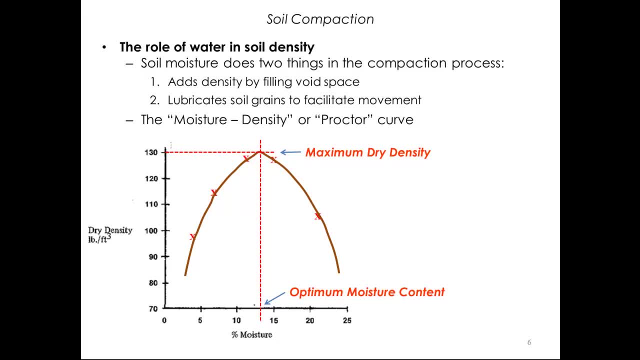 the best combination of soil and water to achieve the maximum dry density and therefore the strongest compacted soil. A good way to help remember the importance of moisture and soil compaction is to think of the two sides of the curve divided by the optimum moisture content line. The left side is 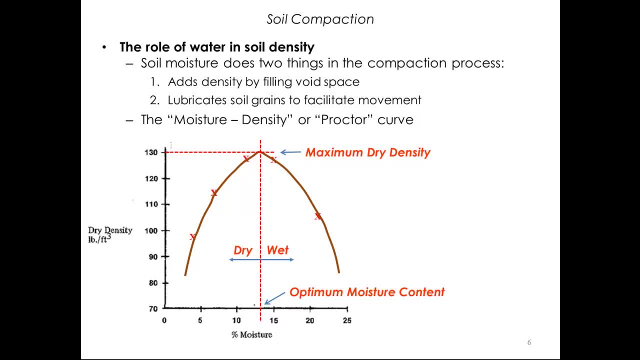 called the dry side because the soil needs more water to achieve its highest density, And the right side is called the wet side, since the soils here have more moisture than needed. Now let's understand how compaction is actually specified. Quick recap of our example. 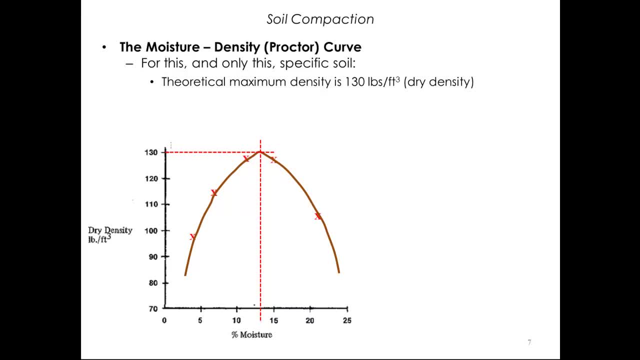 Tells us that the maximum dry density for our soil is 130 pounds a foot and the optimum moisture content is 13%. Okay, so when compaction is specified in our contract documents, it will be in terms of some percentage of the maximum dry density, For example, say 95%. This tells us, and the 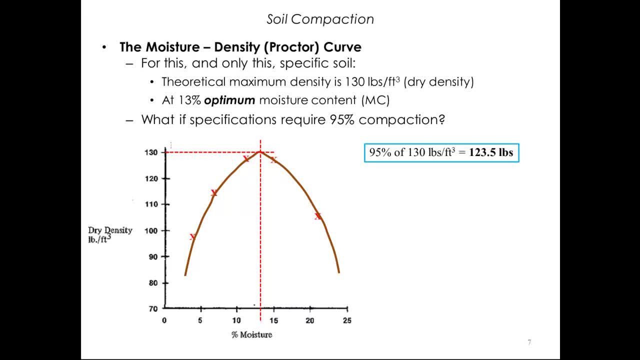 inspector who will be testing the compaction work, that the soil must have an in-place density of at least one hundred and twenty three point five and one hundred and twenty three point five and one hundred and twenty three point five and pounds a cubic foot. If we plot that minimum value as the blue line, here we have defined an. 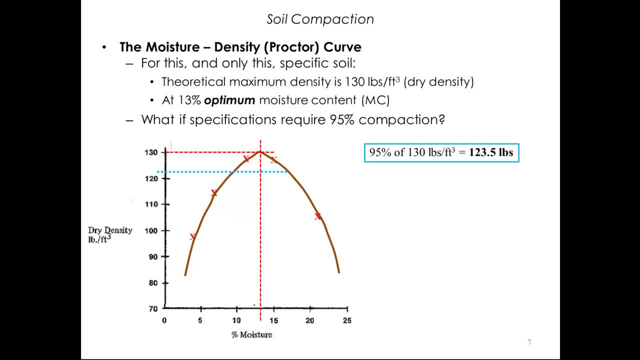 envelope where any field compaction test must plot in order to be passing. that is above the blue line, And if we extend the lines perpendicular, we can quickly see that our soil moisture content must be between nine and seventeen percent for the test to pass. Let's take a look quickly at 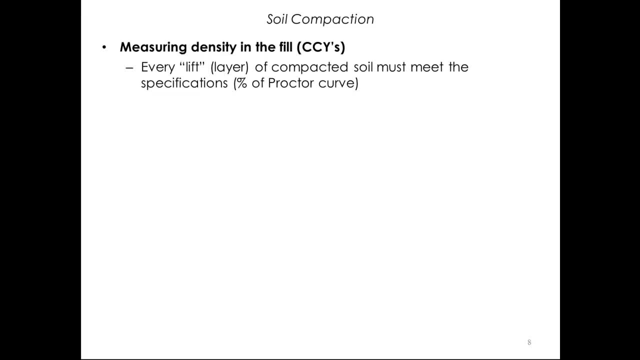 how field compaction is measured. On any project, the compaction of the soil will be measured as each layer or lift is placed and compacted. The usual method is to take one test per lift per five thousand foot of area. Subsequent lifts are not allowed to be placed until 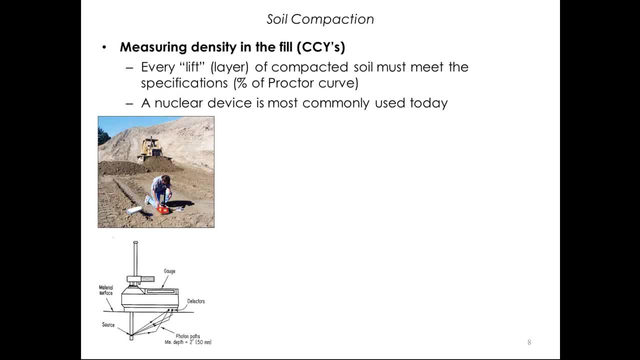 a passing test is obtained in each area. If a test fails, the contractor must adjust the moisture content and or apply additional compactive energy. In terms of field testing, the nuclear device is most universally used, since it only takes a couple minutes to test the soil. If the test fails, the 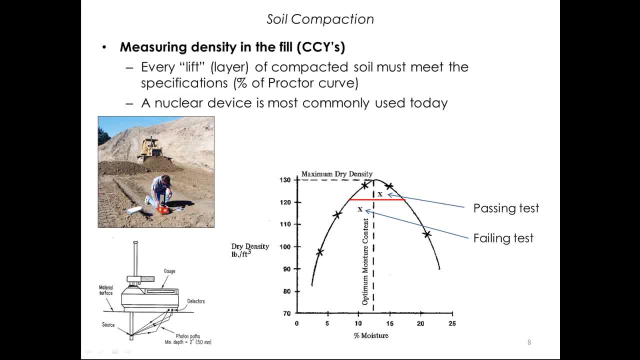 nuclear device is only used for a couple minutes to get the results Illustrated here. then we see examples of two tests that are taken: one test above the line passing, and the other test below the line, which would be a failure.